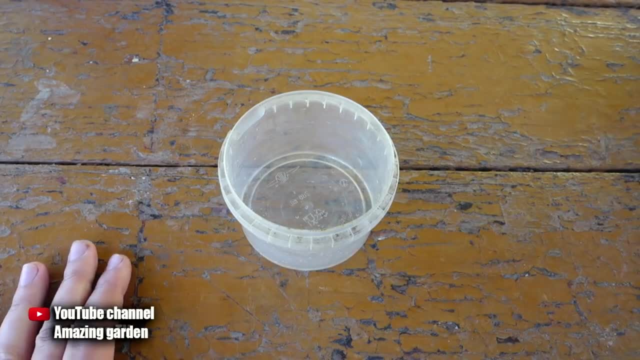 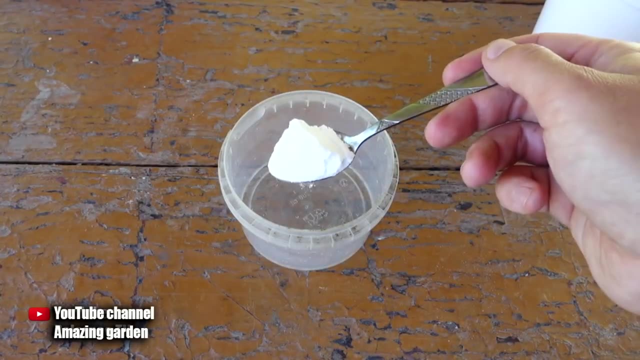 because it will not be possible to use it later. Then we will need sugar, or if you have powdered sugar, it will be much better than sugar. it dissolves much better. To do this, we need one teaspoon of powdered sugar. You will also need hot water. Now I will. 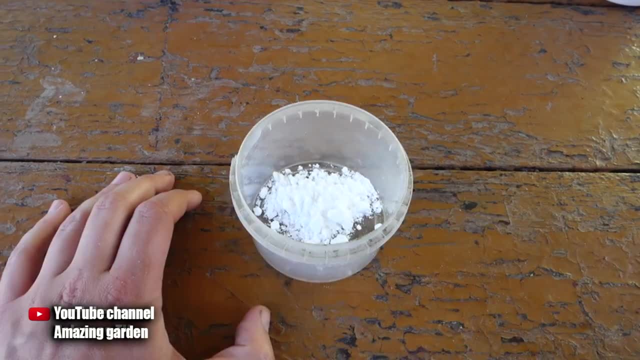 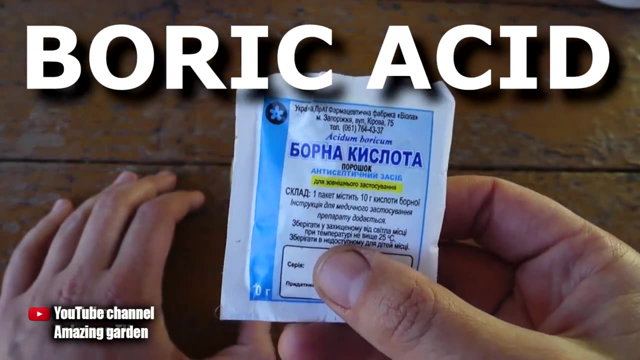 explain why this is necessary. and the second ingredient for our superfood will be ordinary boric acid, which is sold in any pharmacy. it is inexpensive and it is a powder. I thought many of you would have a question: is it possible to use liquid boric acid? Personally, I haven't tried it. 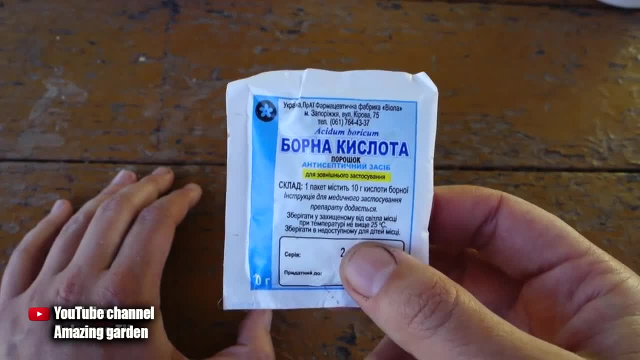 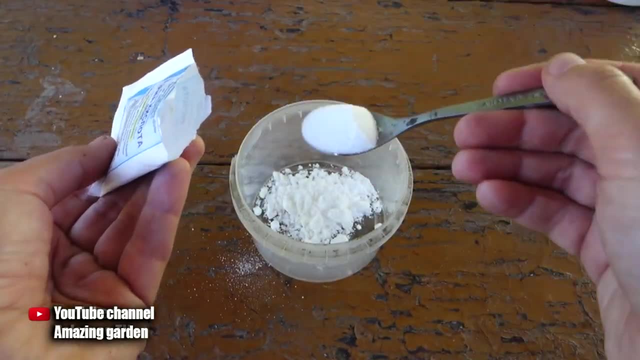 you can try cooking with her. Check if it will work then it's great Write in the comments. I know that dry boric acid defiantly works For one teaspoon of powdered sugar. we will need one teaspoon of boric acid First in the dry. 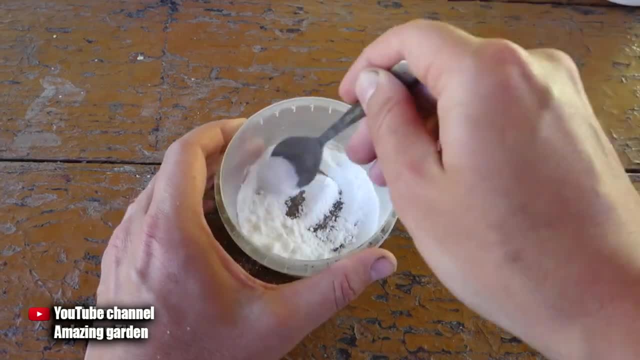 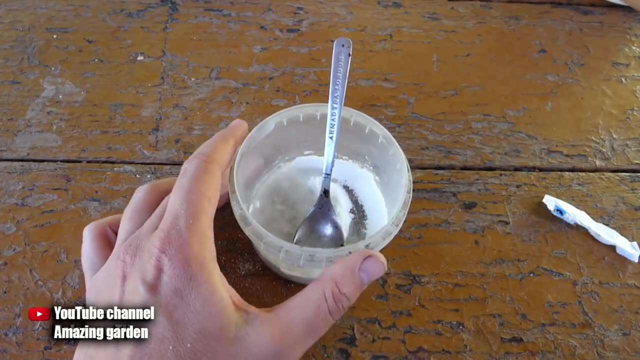 you need to mix it well with powdered sugar. That's why it's better to use it than sugar. The water should be hot. gradually add it. If you pour a lot of water, then you can add both boric acid and powdered sugar. That's actually. our bait is ready. It will need to be kneaded. 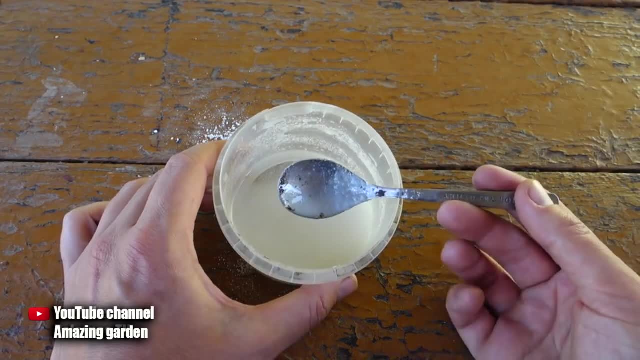 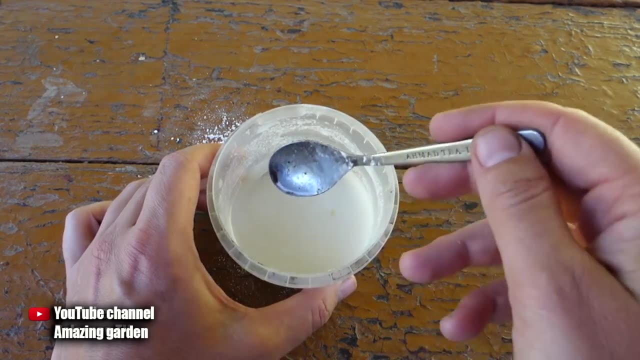 to a consistency that resembles thick jam. This is a great density, because we will then put this in the oven and let it dry out. Well, ants can do anything, and they really like sweets. Now let's go to the garden. I'll show you how to properly install this bait next to the anthill. 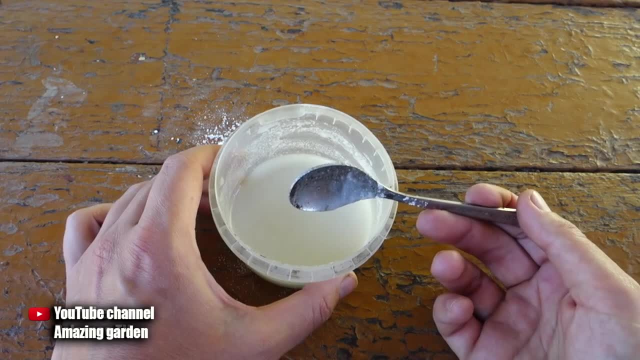 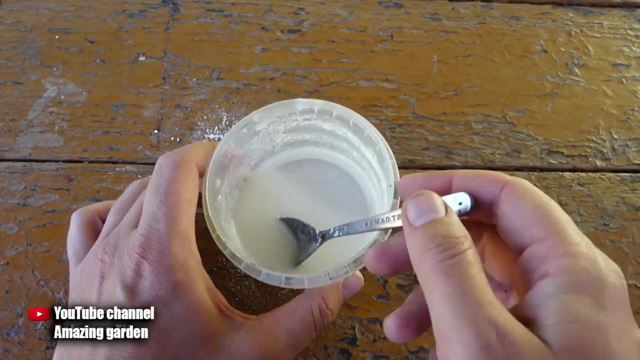 But of course I also want to make a small warning. This bait is also dangerous for pets. if you have cats, dogs that you often have in your garden or where the anthill itself is located, then such a bait will need to be covered with something heavy Ants will find an. 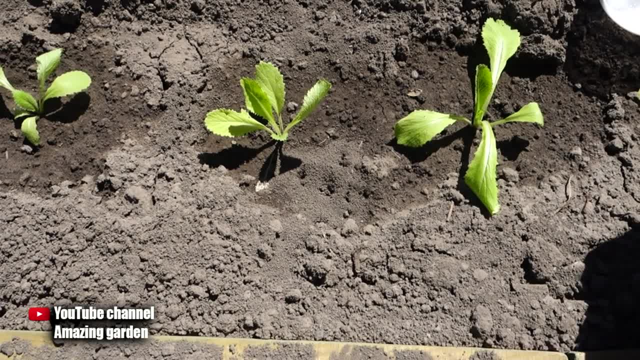 approach to it because they are small. The main thing is that your pets cannot eat it. it is also desirable that children do not touch this bait. It is desirable to put this bait in the morning or during the day, but not in the evening, because at night the activity of ants decreases and they 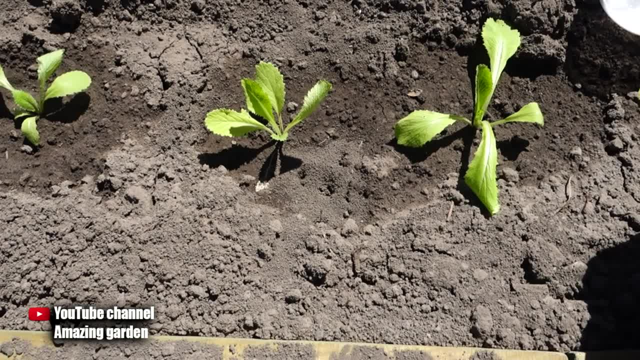 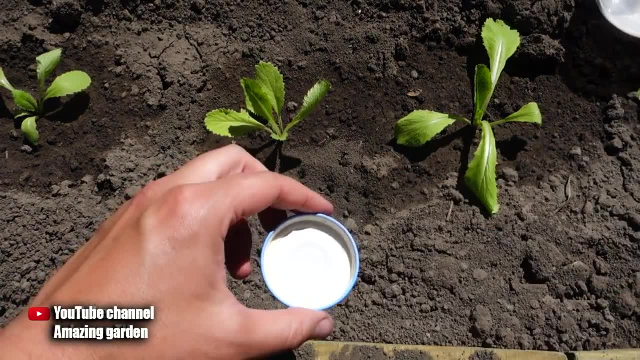 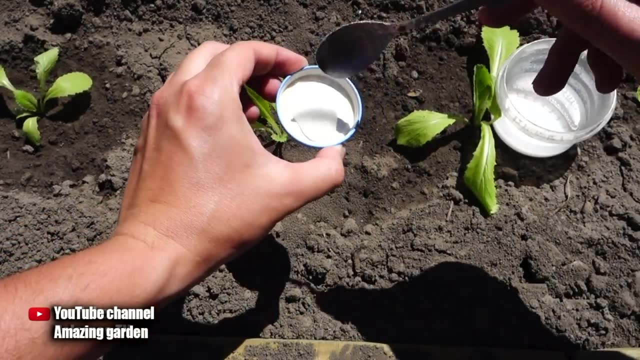 go into the anthill itself. We need to establish, at the moment when the most active phase of their work is underway, What are we doing? We take the bait itself: a small lid, preferably something, so that there is a small side, So that our bait does not spread. we put one spoon here And we install.